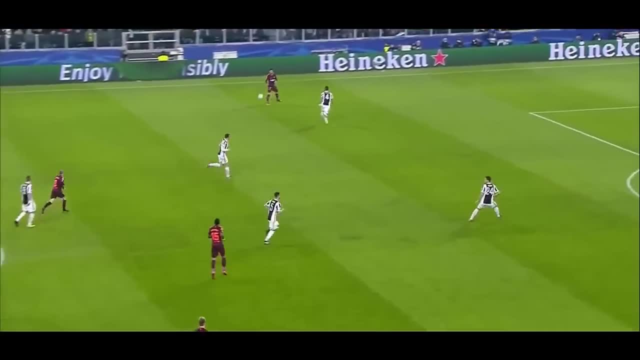 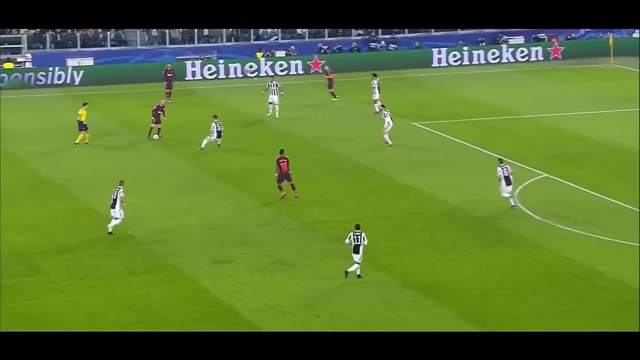 on the attack. you can see he doesn't delay too long. he assesses his options. no one is really closing him down and he picks out the pass very nicely. in this play, again, you can see he's assessing his options. no one's really going in on him and he decides just to keep possession keep. 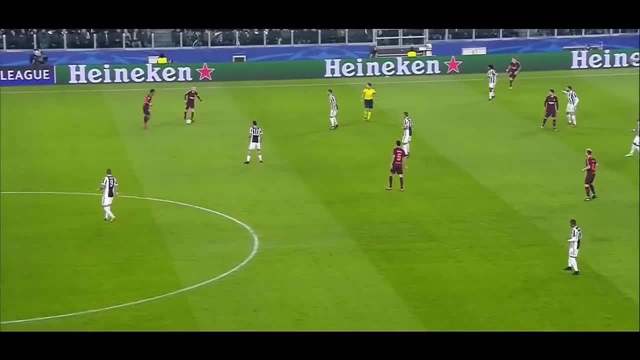 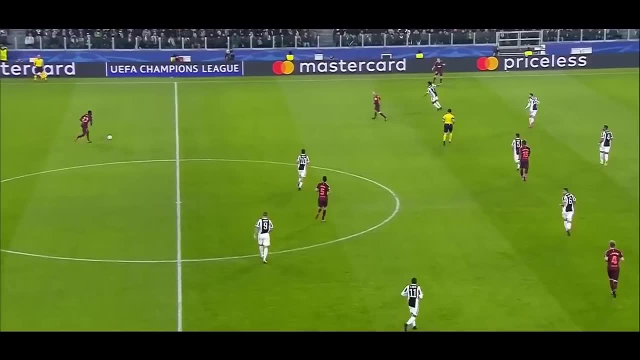 the ball moving again. he does something similar in this play- not going to really break it down any more than that, because it's essentially the exact same thing. he does again here. he is checking for the ball and his awareness is good here, and he sees that the Juventus player is backed off him a. 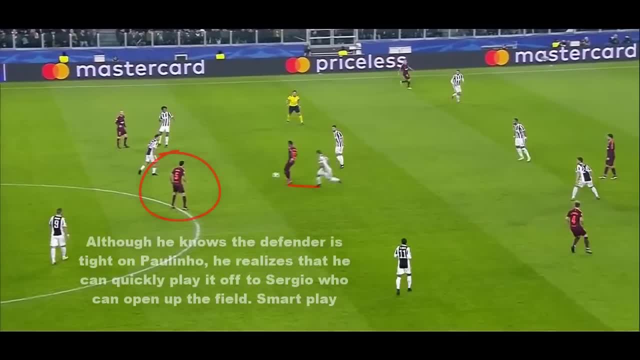 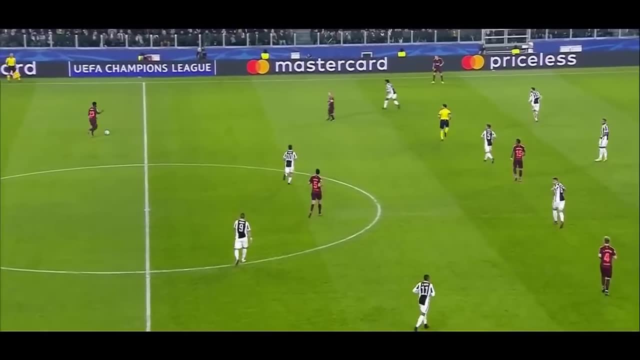 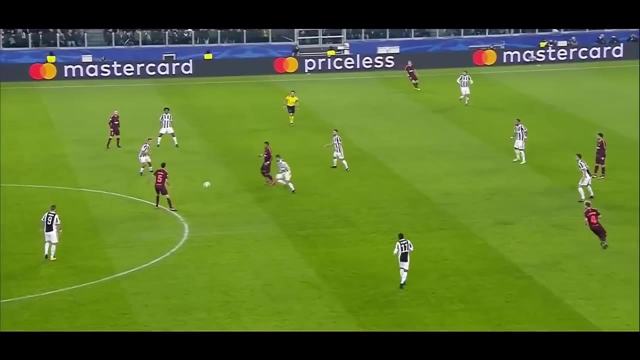 little bit so he's able to turn and he immediately plays a forward pass quickly, playing quick, not allowing things to be delayed. at this point, Barcelona don't really make too much forward progress here, but it's a good idea by Iniesta and again notice how his awareness allows him to know how close the Juventus defender is to him, which 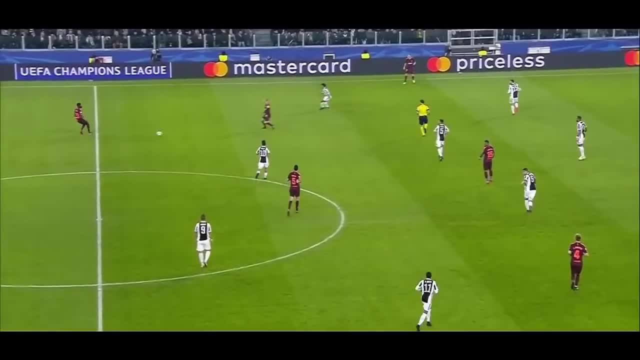 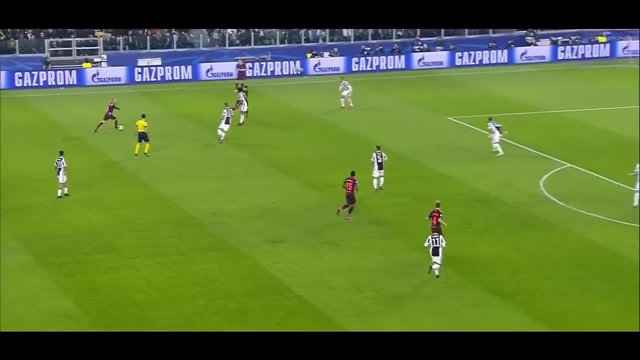 allows him to turn, where if the Juventus defender was right up on him, he may not have received the pass in the first place or would have played it right back to the passer. so in this play he gets the ball again and he notices that he has men forward. so he moves the ball forward, drives. 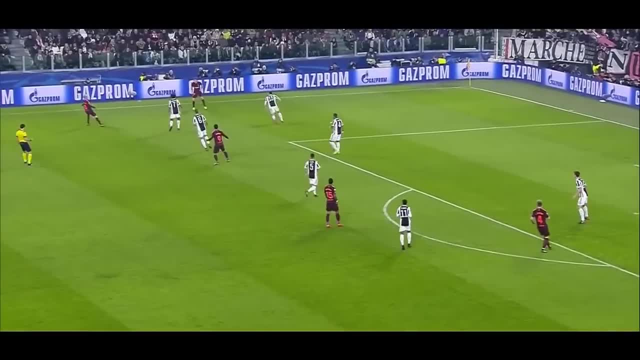 forward and, of course, he just plays the ball right out to out wide and gets the ball back again. he's looking forward and plays a really good cross field ball to switch up the ball and he's able to turn, and he's able to turn, and he's able to turn, and he's able to. 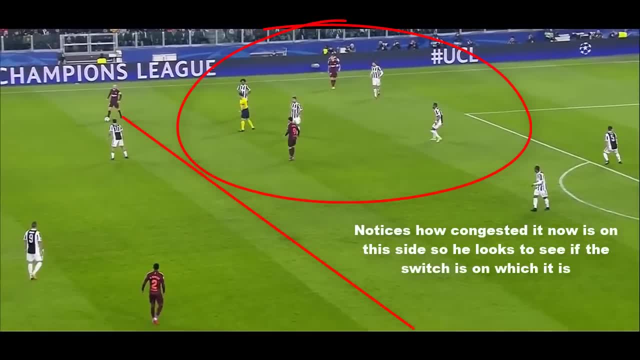 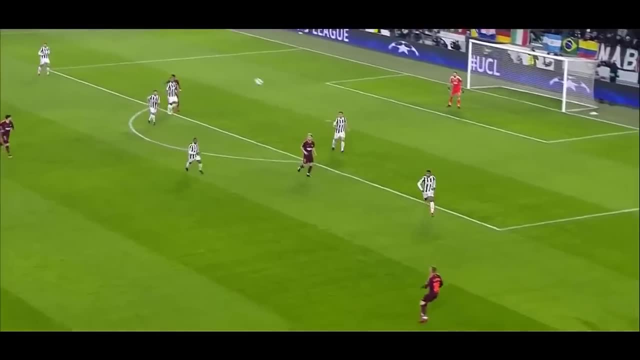 play because it was getting congested on the side. he was on. but again, this is good, because in the other plays he didn't move forward because he didn't really have too many people with him- there weren't too many people in central positions- but here he does try and go forward. he switches. 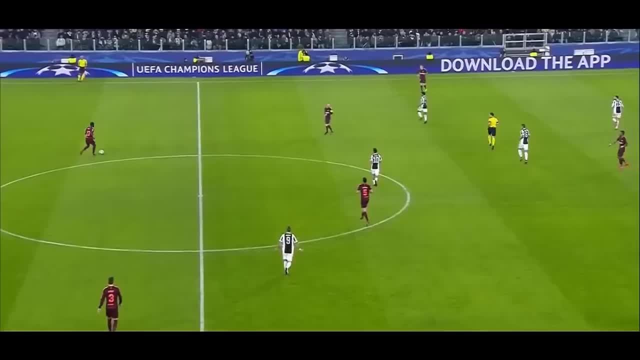 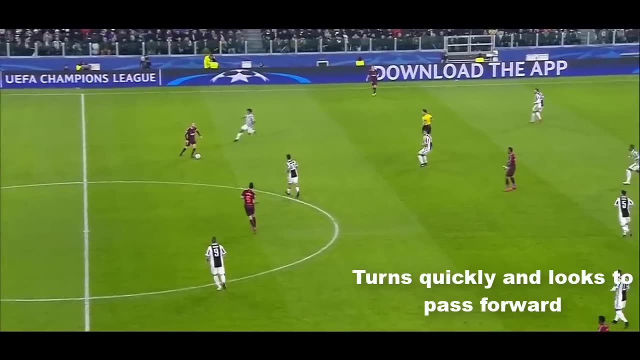 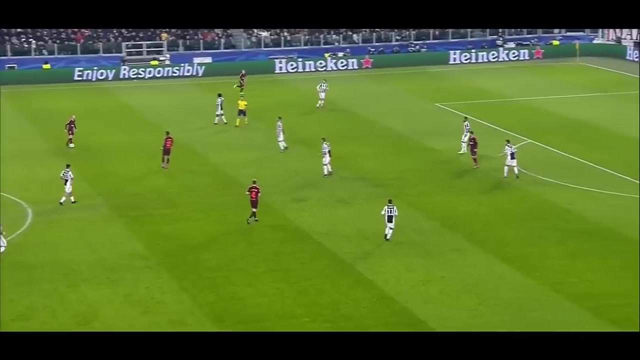 the play and it's very positive play by him. here again he checks back to the ball and tries to play a forward pass, getting the attack going. not much comes out of it again, but the idea, once again, is right. here he gets it in plenty of space again, trying to go forward, but he's taking his time, he's delaying, he's keeping. 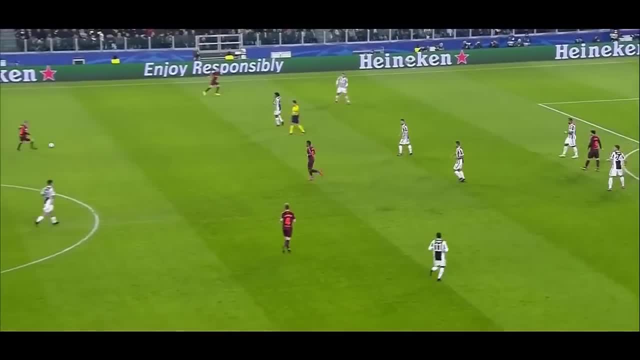 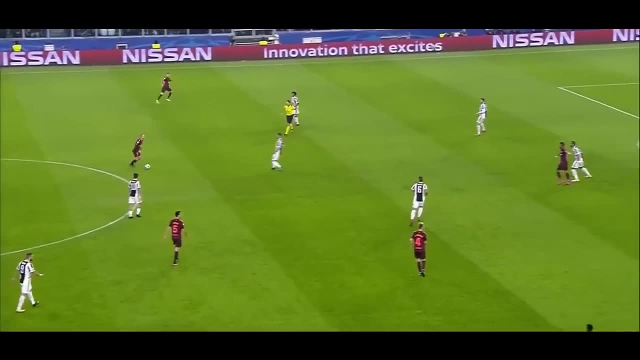 possession and eventually passes it back when he doesn't have much option. again, he's not forcing anything, he's being smart in this moment. so now he gets the ball in plenty of space and again immediately tries to move forward, plays the forward, pass again. this is the right idea. it. 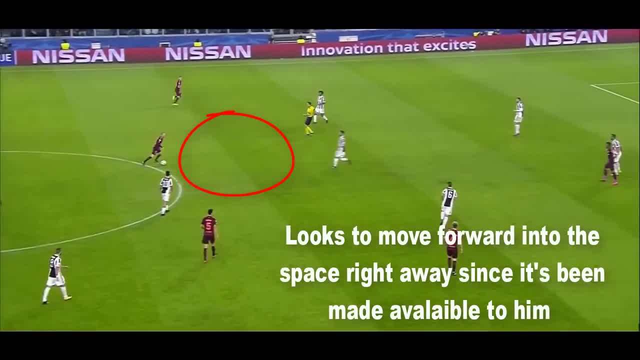 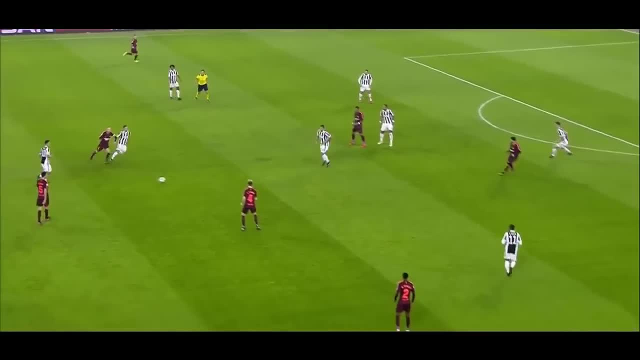 looks like his pass is a little bit too far in front of Rakitic, but again you can see, when he has that space to move forward, he will take advantage of the space the defenders are affording him. again he gets the ball in a pocket of space. he's checked back for it and he just keeps it moving. 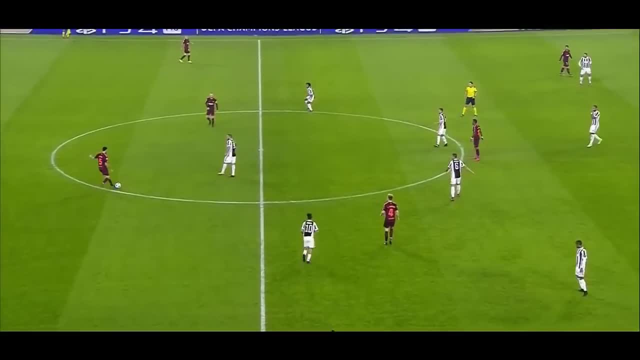 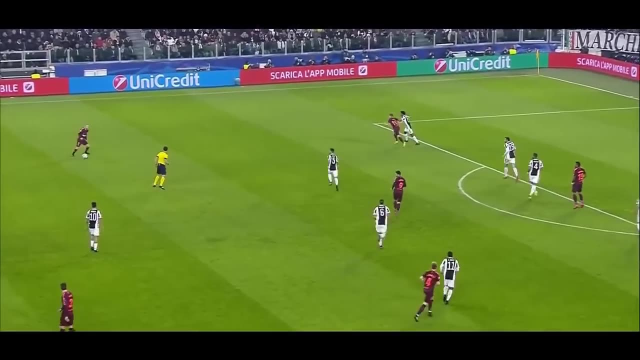 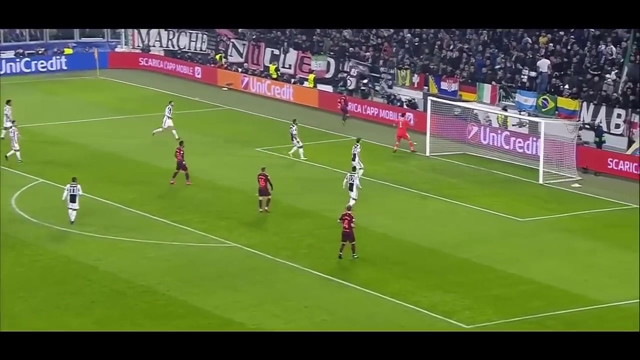 along by playing it out wide again. a big part of Barcelona's play, or the way they play, is they like to keep the ball moving, again available in plenty of space, and he immediately goes forward, plays the ball forward. it's not a good return ball, I believe by Suarez, but look at the anticipation by him. 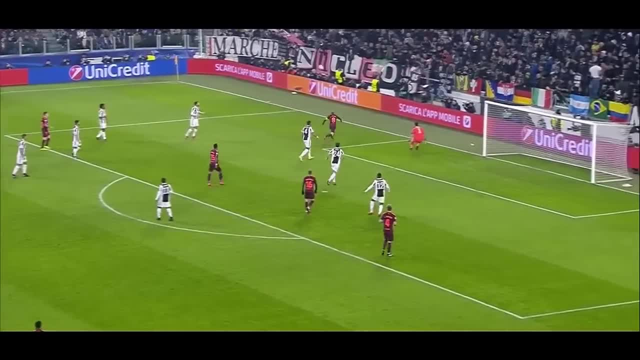 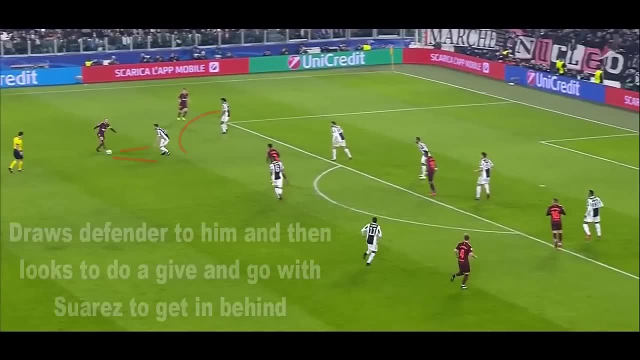 for the backwards pass. he's anticipating what the defender will do, looking for any kind of mistake, and it's really a great play from him, even if the return is a little bit too far in front of him. ball wasn't what it needed to be. he was looking for that quick give and go and if you look, look at it, 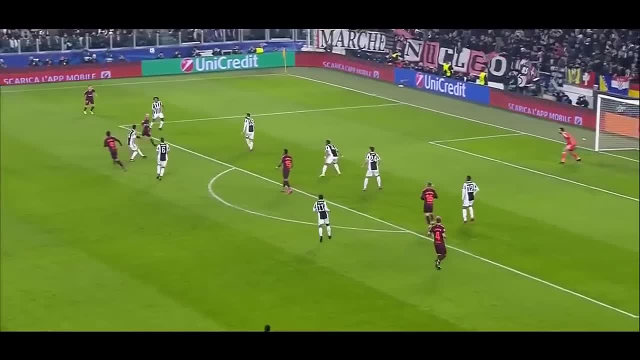 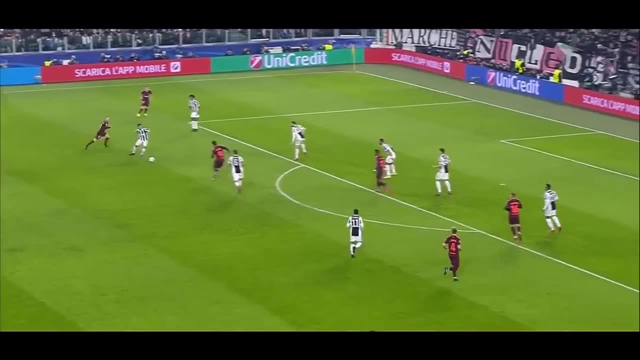 if Suarez just plays the ball back on the floor or to him, he's probably going to get it back in a good position. but again, look at the way he drives at the defender trying to make things happen and notice how, when he gets in those huge amounts of space, he takes advantage of them. 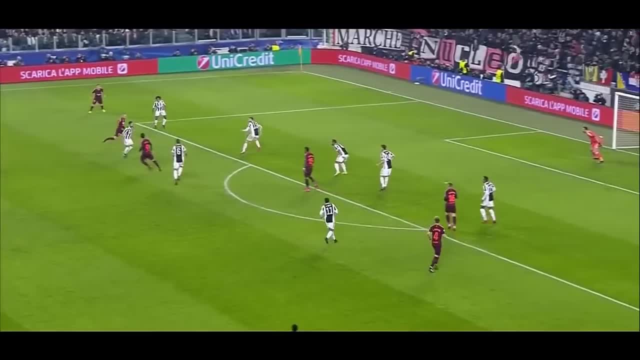 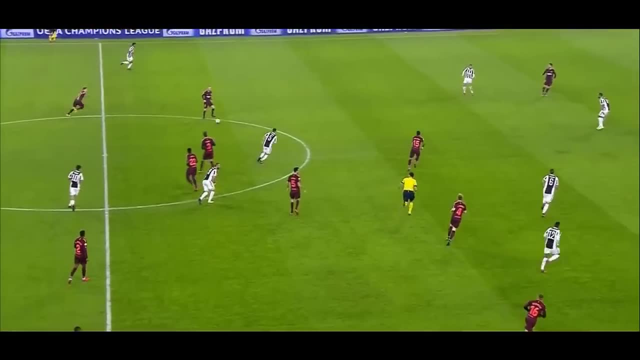 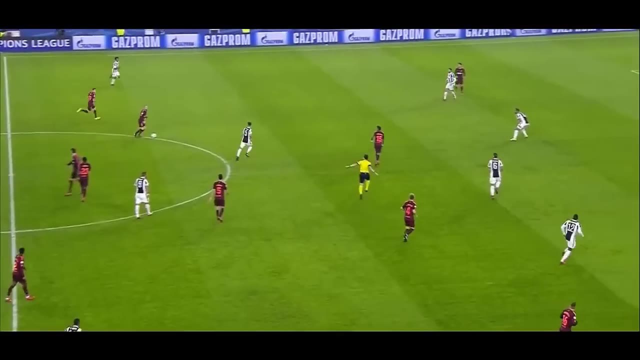 by driving forward and putting the defenders under pressure. here he is again. in plenty of space. he's assessing his options, plays a simple ball to keep it moving. take too much advantage of the space here. he doesn't run right into it. he could have probably drive driven right into that space. it's not really a mistake, maybe just a better decision. 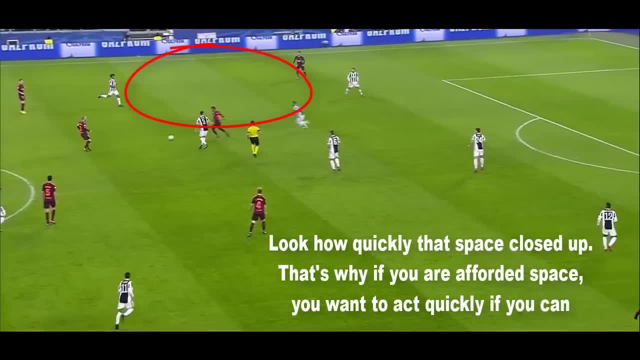 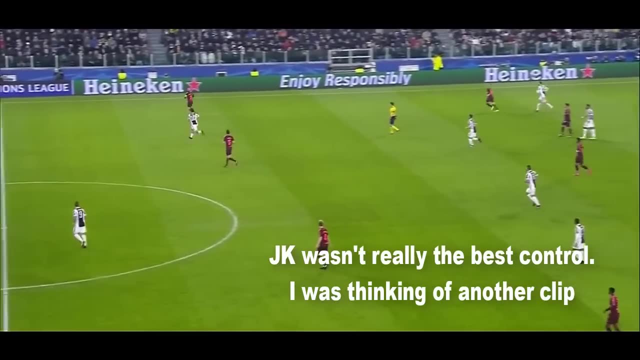 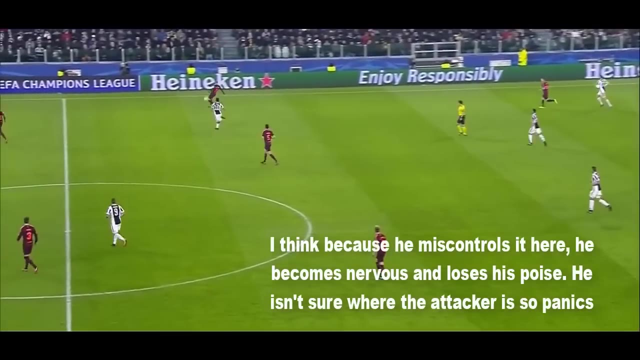 he could have made, but again, he's trying to keep the ball moving, trying to get other players involved, so it's not really a bad play. so here, excellent control by him, but he makes his first mistake of the game, which is very rare for Iniesta to make this type of mistake where his awareness. 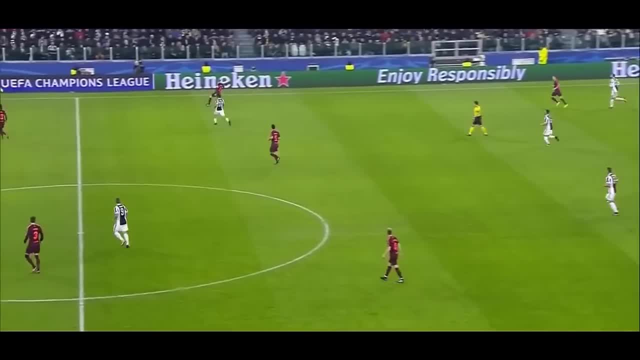 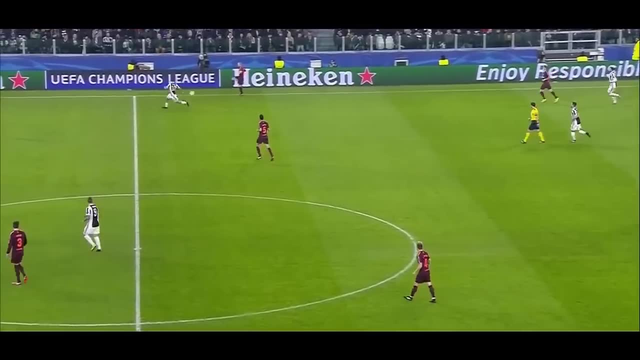 just wasn't good. make sure when you're playing in this position, you know where opponents are and you know where your teammates are. i don't know if he thought someone was on him and he needed to play it quickly. he didn't know where the opponent was and he ends up playing it. 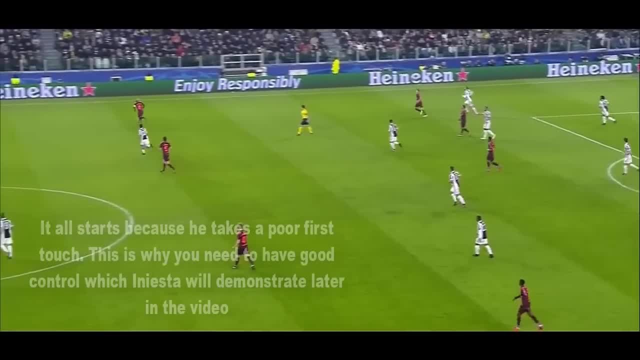 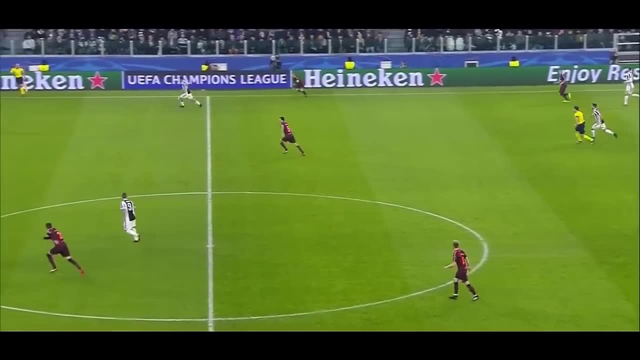 right into their path, and it's a rare moment of panic for Iniesta, something you don't usually see in that situation. it would have been better for him to make sure he knew what it was around him. bring the ball down to his feet and he would have realized he had plenty of space to then. 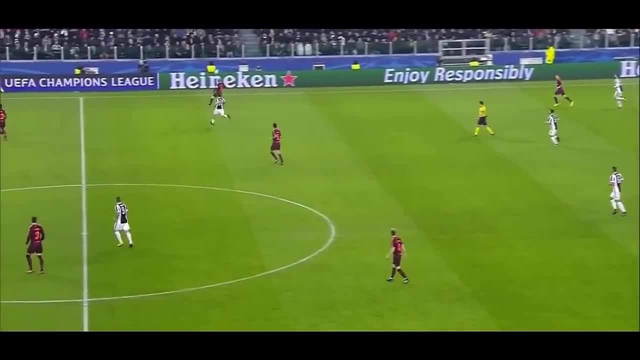 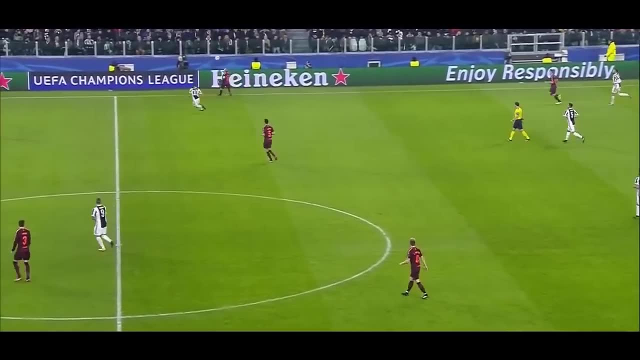 actually go forward. so first mistake by Iniesta. but just take away from this. you want to know where everything is at all times, because if he was just aware of where to play it was, he wouldn't have made that mistake. so here, great play wins the ball and look how he. 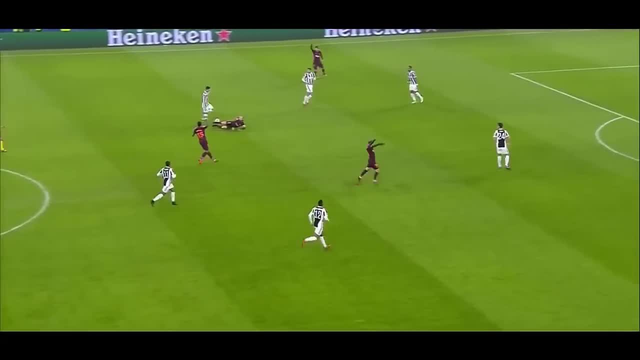 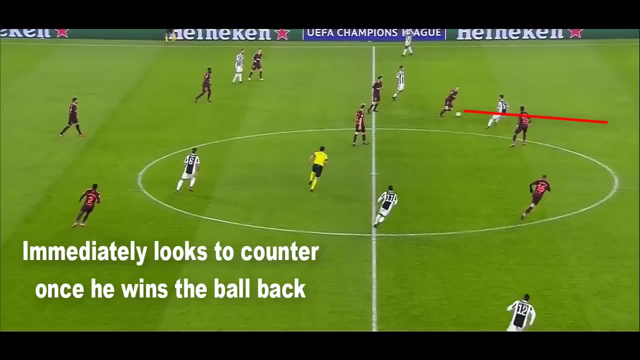 immediately tries to go forward and then gets tripped up, which i would assume the defender got a yellow card for again. so many good things he did here: one winning the ball back, pressing high up the field and winning it back. it's a great tackle. and then look how he doesn't delay. 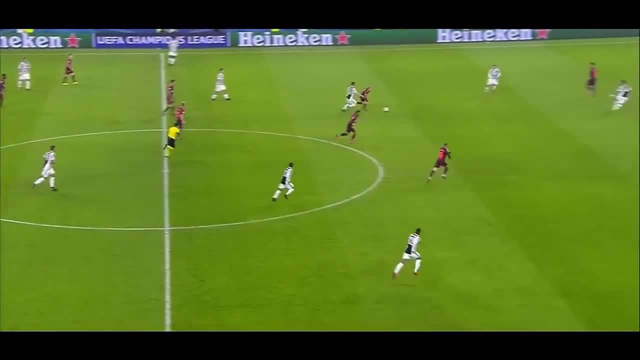 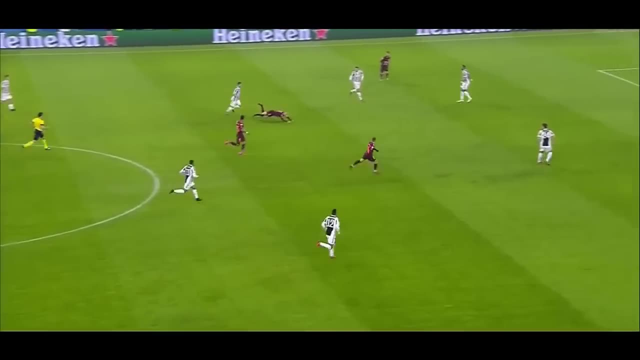 he immediately sees that he has his own players in the attack and tries to go forward, does really well to move past the defender, and this is why you know you want to pick up the ball and you want to penetrate the defense. you want to run at them sometimes, because now not only do they get a free, 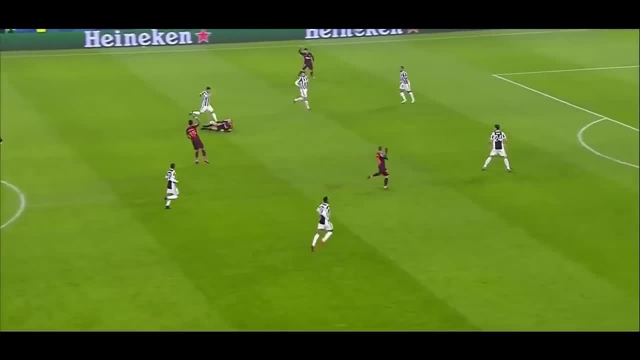 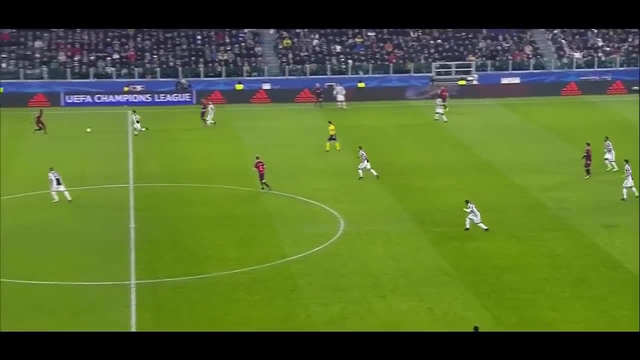 kick in a dangerous position, but now the defender is going to be on thin ice by receiving the yellow card, so here gets the ball a lot of pressure on him, so just plays it off again. sometimes you just need to play simple. he does a good job of getting his body between the ball and the man, but in these 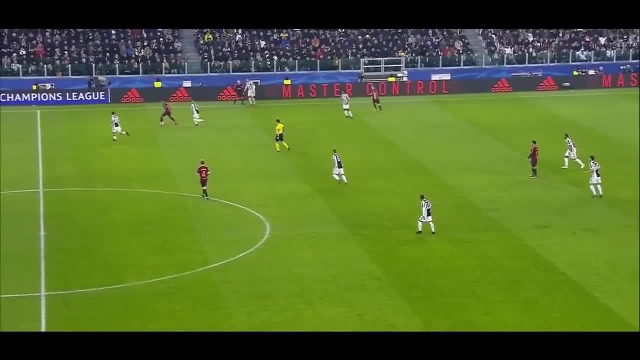 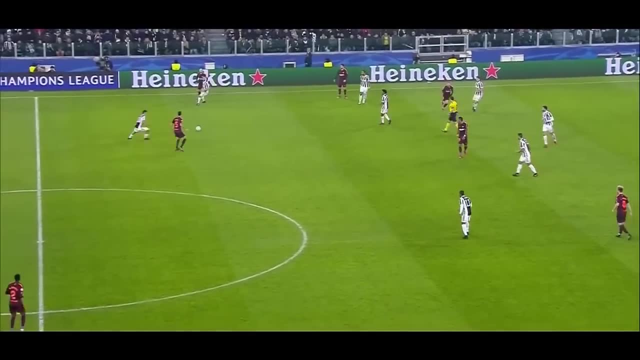 situations. no need to risk anything. defender's right on him doing a good job, so he just plays it safe. okay, here he has a little bit of space, plays it out wide. he look how he immediately takes a few steps out wide to create the passing lane. so his teammate. 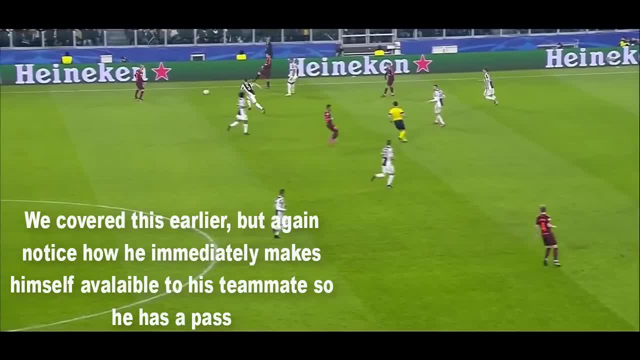 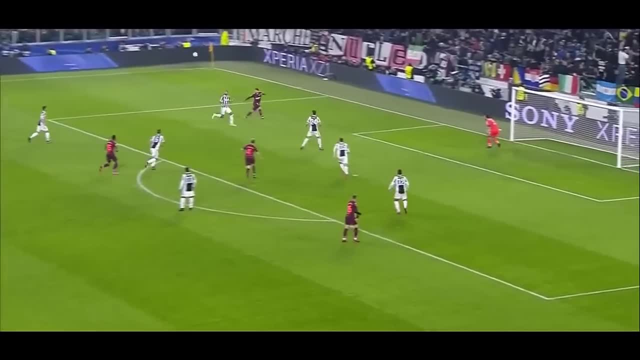 can play it back to him. another thing: you need to make sure you're doing passing and moving, passing and then getting into a position where you can receive the ball back. so here he makes himself available again and tries the give and go again. good idea. it's a very hard play to make. 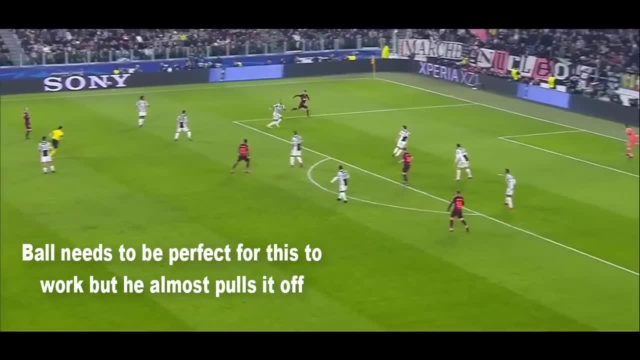 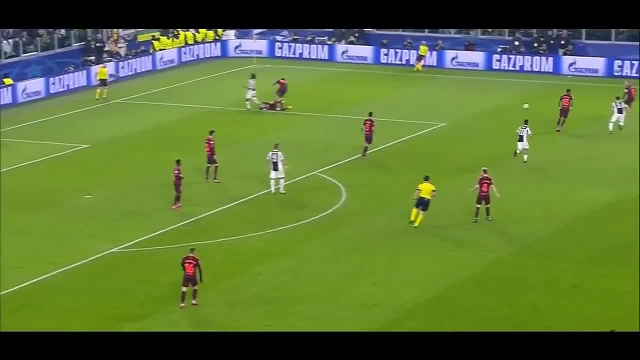 because there isn't much space for him there. if he hits it too hard, it goes out of bounds. if he hits it too soft like he did, it's cleared away. but it's the right idea. it's very positive play from iniesta. he's going to get the ball. he's again. he's assessing his options. he sees that he's. 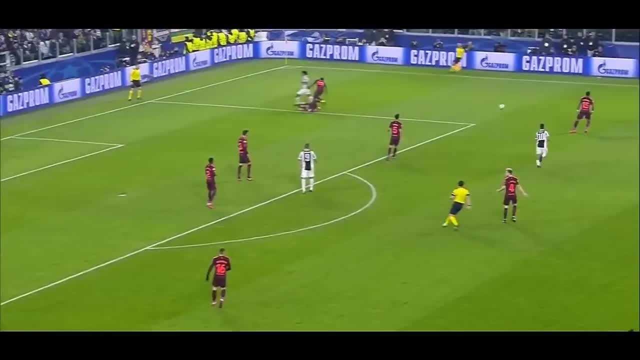 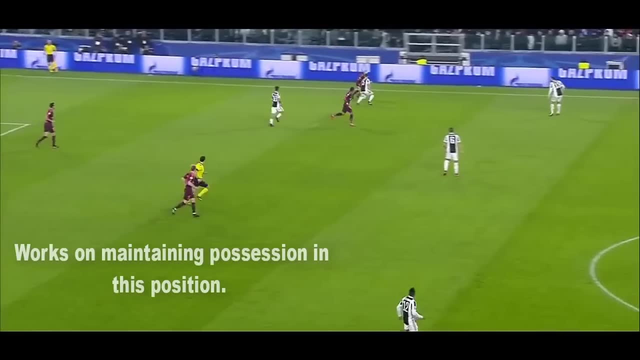 basically being played out wide and he doesn't have too many options forward. so he plays it safe and it looks like barcelona got free kick anywhere. but just kind of look at what he does. he realizes maintaining possession in this position is going to be better for his team, so he cuts it back and 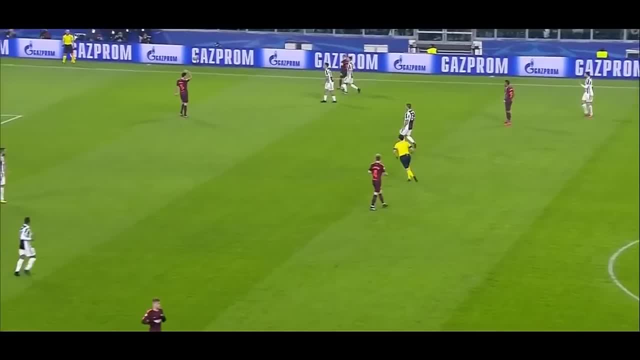 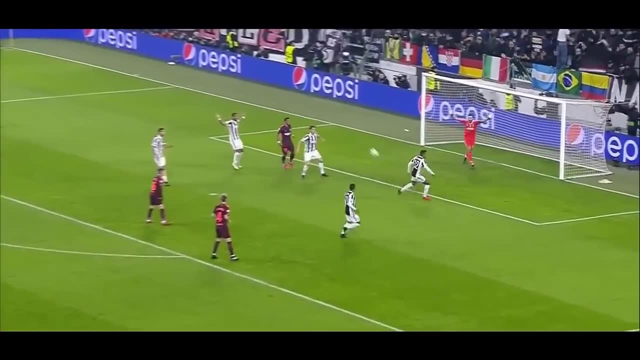 if the foul wasn't called i'm sure he would have played biscuits in that play. so here he is. he's making himself available out wide, assessing his options again, but really quickly, doesn't delay, puts in not the best of crosses. but he only really had suarez in the box so he didn't have too many. 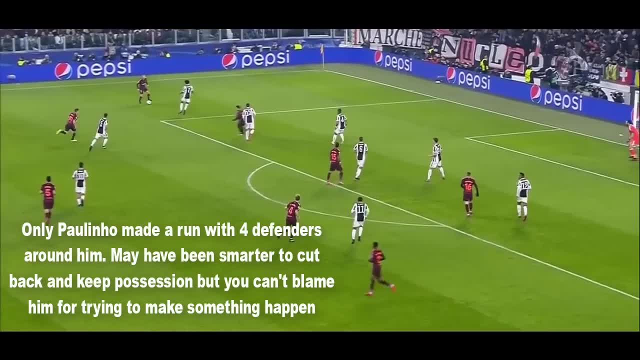 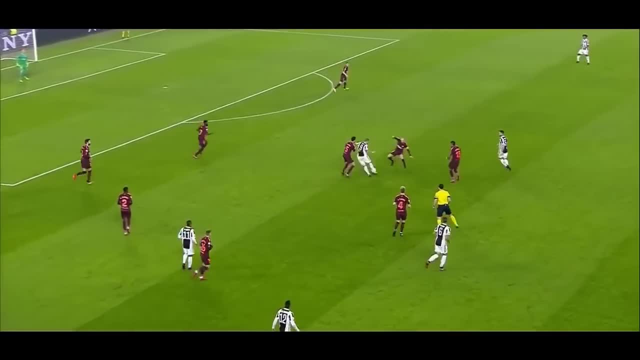 options. again, not a bad play by him. he immediately is trying to be positive, cuts it onto his other foot and tries to put in the cross. here he is with another great tackle, great defensive play, gets the ball back and this is a really great play because of his awareness. he knows that. 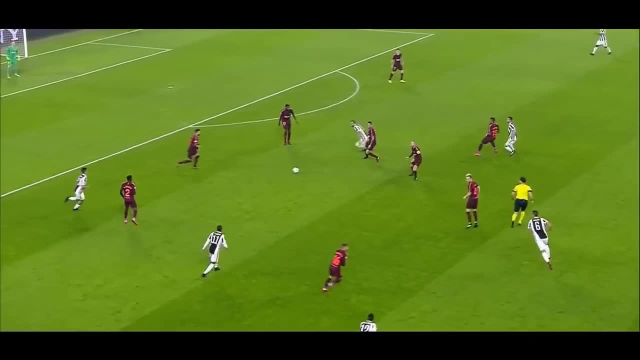 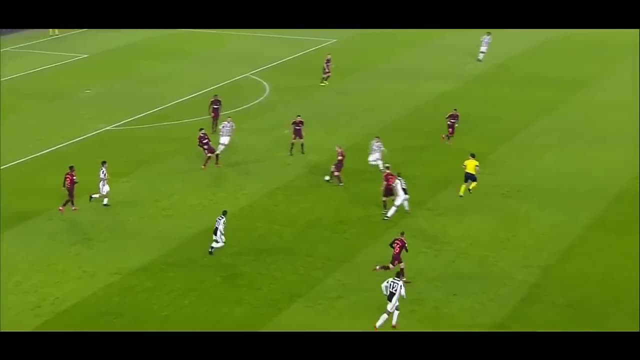 immediately after winning the ball, juventus is going to press, press, press the defenders- which they do um- and he plays it to the defender, who plays it right back to him and he's aware that two players are moving in on him and he knows where his teammate is. nice little flick. 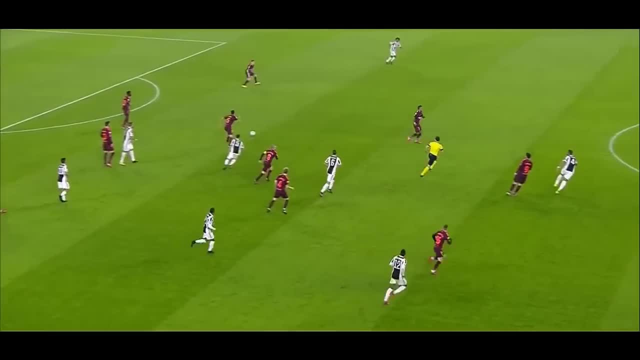 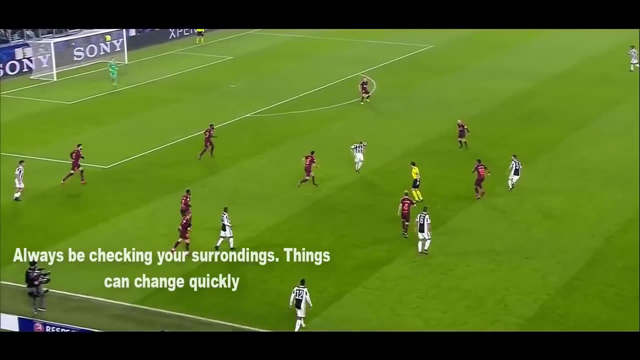 of the outside of the boot and they could have potentially countered from that position as well. so, again, this is just another me reiterating how important your awareness is and how quickly you need to become aware of your surroundings and the ever-changing surroundings in the game, because 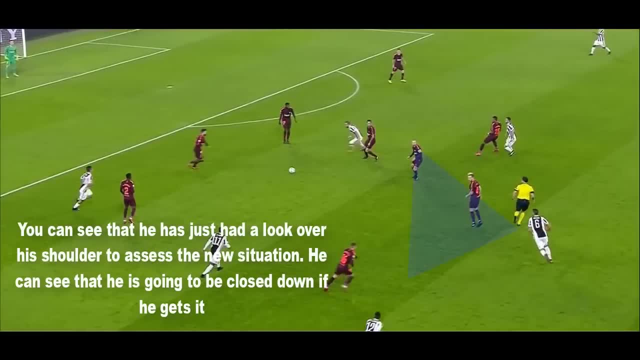 again. he wins the ball back and immediately has to make sure he's aware of what's going on around him. he can't turn off because if he does he's going to lose the ball. he stays focused, notices the defender's kind of collapsing. he's going to be able to get the ball back and he's going to. 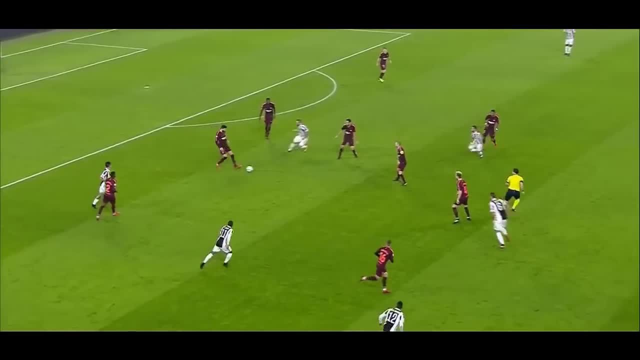 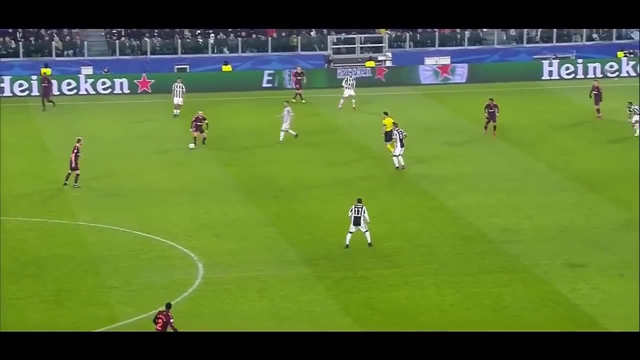 just be relaxing in on him and again is able to beat two defenders, essentially take him out the game with that little outside of the foot pass. here he gets the ball in plenty of space but realizes again that he's going to be closed down quickly and plays a simple ball to rakitic here. 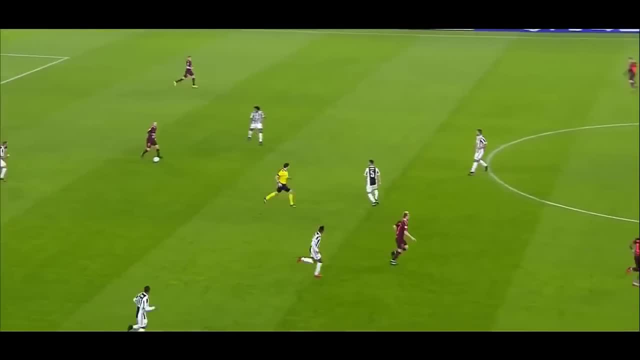 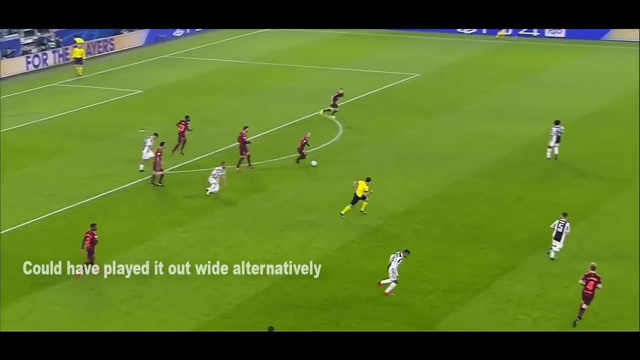 he's taking it out of the defense, assesses his options, doesn't have much, and draws the foul, which is actually a good play to relieve the pressure, having just won the ball back. i do think he could have played it out to the left here, um, but in all honesty you know there wasn't a bad play, really by. 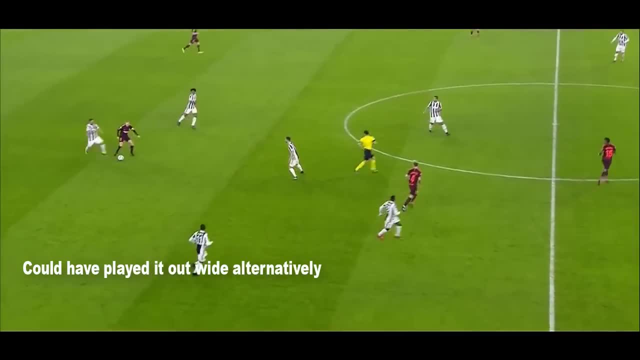 him. but you can see he's got a lot of control on the other side of the field and he's playing really well in the second half of the second half. he's got a lot of control on the other side of the see if he could have played it out left, but quadrado kind of takes that away from him. 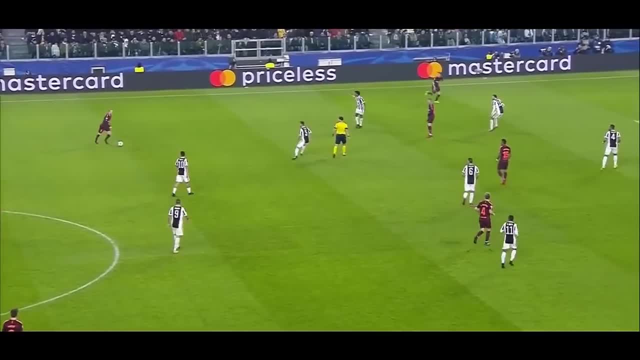 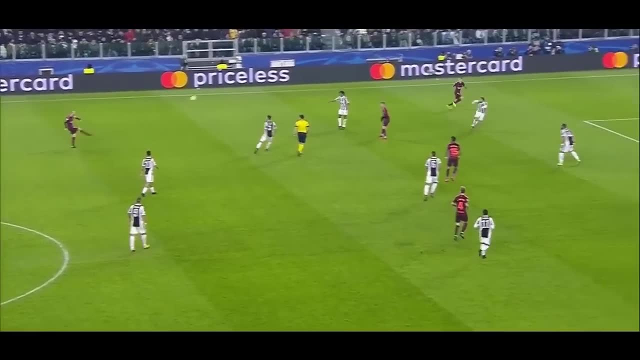 here he's getting it in plenty of space again and he plays a really good ball out wide again, keeping the ball moving very quickly. he could have driven into the space, but he noticed the run and wanted to take advantage of it to put his teammate in closer towards the box and i think 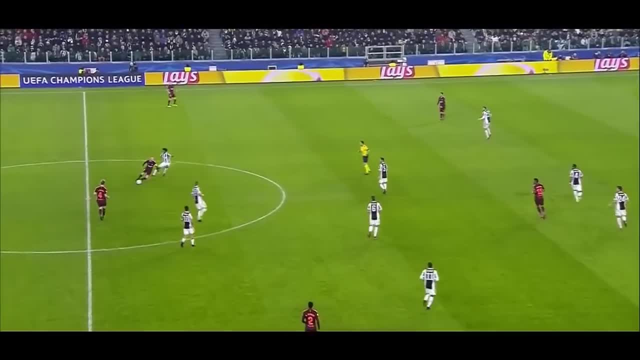 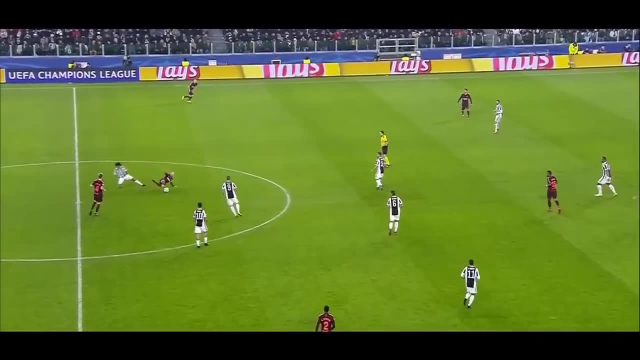 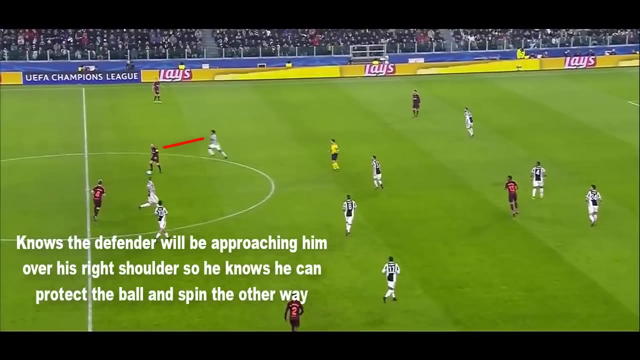 this is a good play as well. here again, he notices the defender coming in really quickly and does really well to swerve kind of around him. he notices which angle the defender's coming from and, you know, keeps the ball close to his body and draws the foul. this is something that inies is. 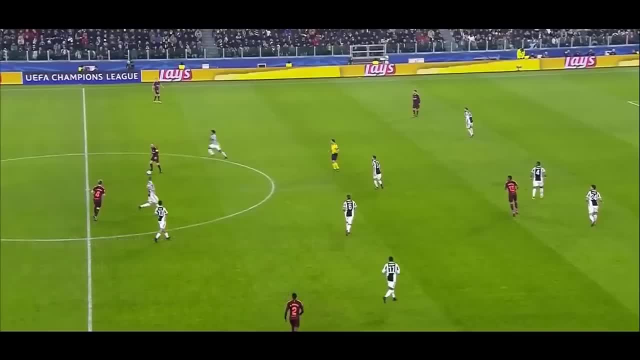 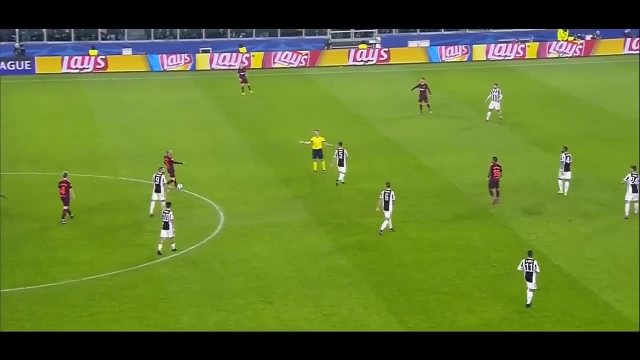 so excellent at protecting the ball, keeping it close to him, and if he wasn't fouled there he would have had so much space to move into, as you can see with his frustration when he doesn't get the advantage. so again, he's afforded a lot of space and just plays it out wide. not much to go. 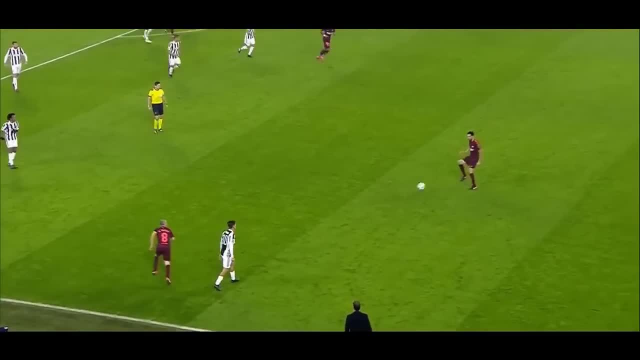 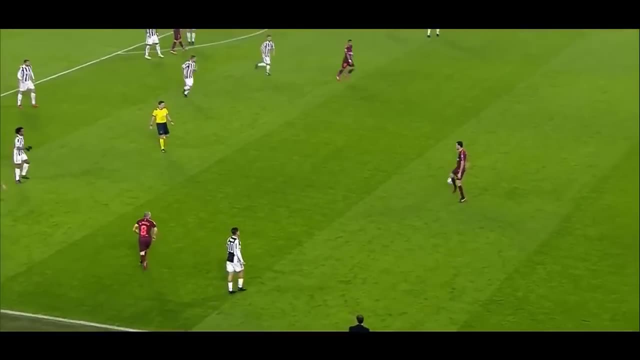 on there here he takes an excellent touch and then plays it quickly. you again, as a center midfielder, you need control like this, because if he doesn't take a good touch there he's going to be closed down. but because he takes an excellent first touch, you can see he's able to play two touch football here: one touch to bring the ball out of the air and 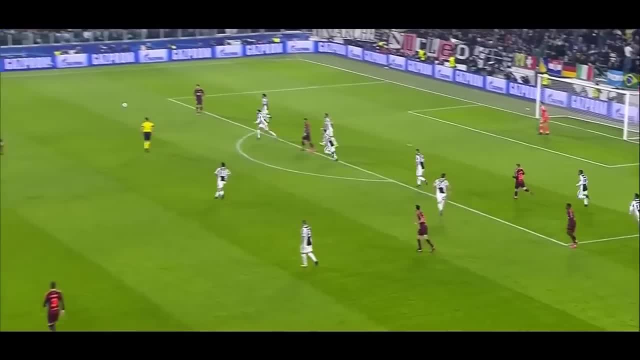 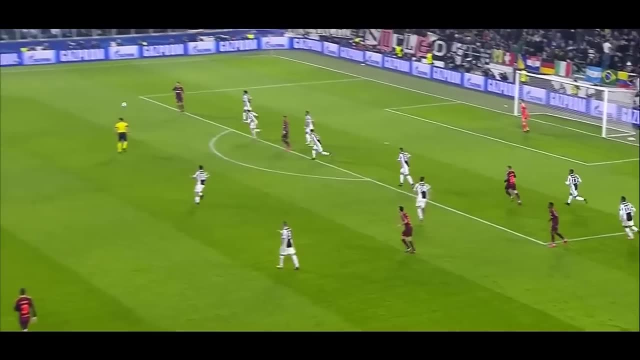 then another touch to pass it off to busquets. so here good control again assesses his options, and i really like this play because he notices the middle is very congested so he cuts the ball back out wide, seeing if they can attack from a wide position again. this is a very subtle thing. 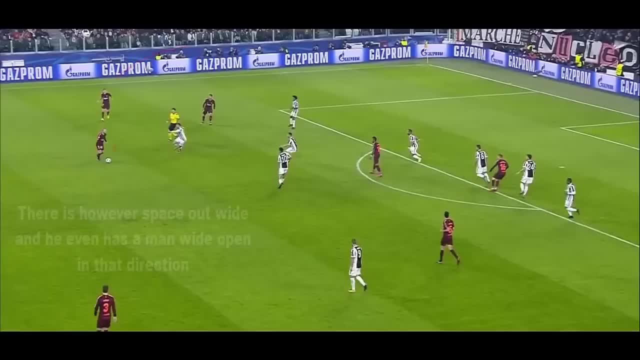 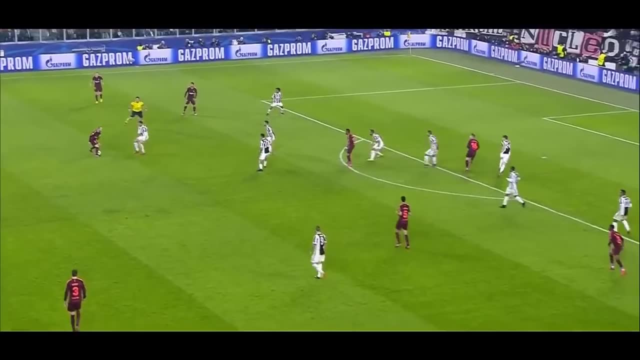 but it's very smart by him. if you look at where his teammates are, they're all really covered in the middle. it's congested in there. so he makes it look like he's going to go to the middle, cuts it out wide, protects the ball and then barcelona have a little more space there again, very underrated. 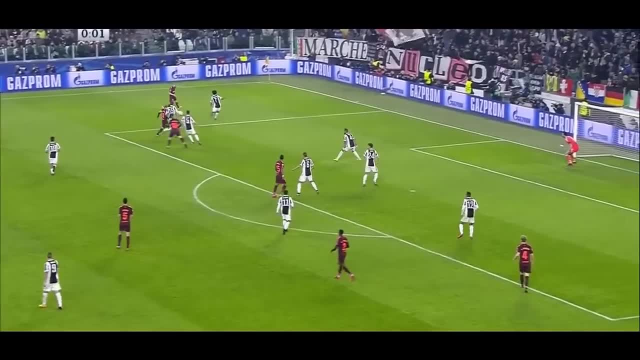 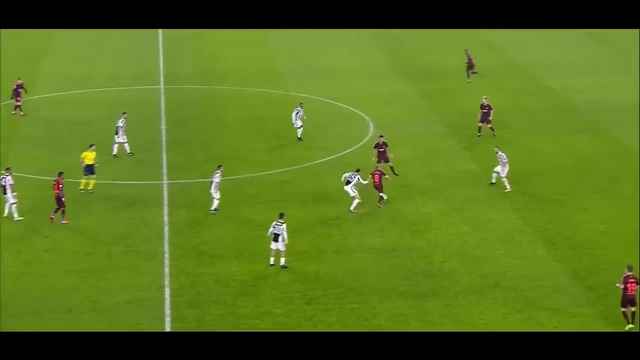 play, but subtle and very good play and smart play by iniesta. so second half iniesta gets the ball, protects the ball. the defender actually does a very good job on him, but then he switches the play. good play all around here, he gets it in more space and then he's able to play the ball back to the 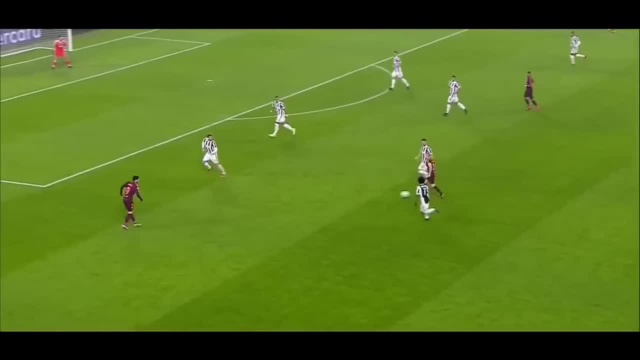 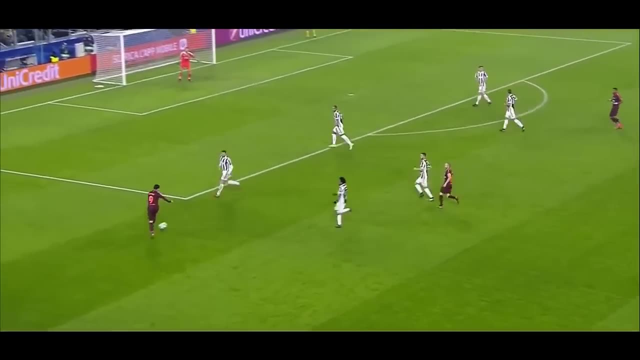 defender and watch as he drives at the defender and then plays it out wide to suarez again. he sees the space. he draws the defender towards him. it creates the space for suarez out wide- another good play by him. so here he gets the ball and this is an excellent touch- and then draws the foul. 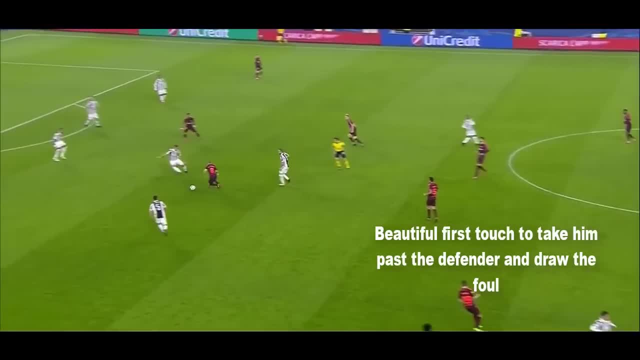 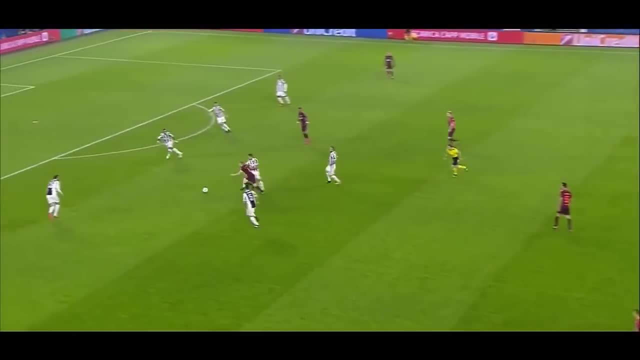 again, just attack minded positive. he notices he has a player out wide. i don't know if you can see him, but suarez is out wide, meaning he can take the ball forward and if he's closed down he can play it off to suarez here again in plenty of space. you can see he's dropping deep a lot more. 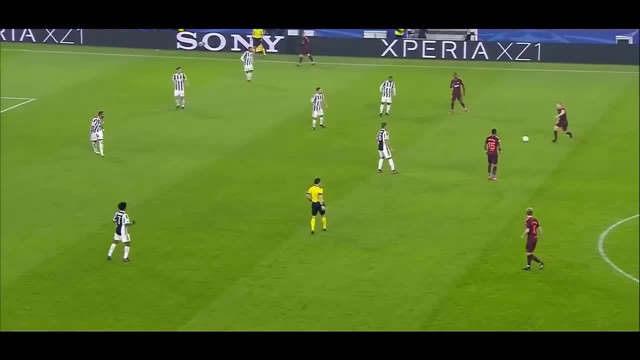 switches the play and then he's able to play the ball back to the defender and then he's able to a wide open player- something you're going to want to do a lot as a midfielder- and when you have a player that wide open, with that much space which will allow them to run at the defense. 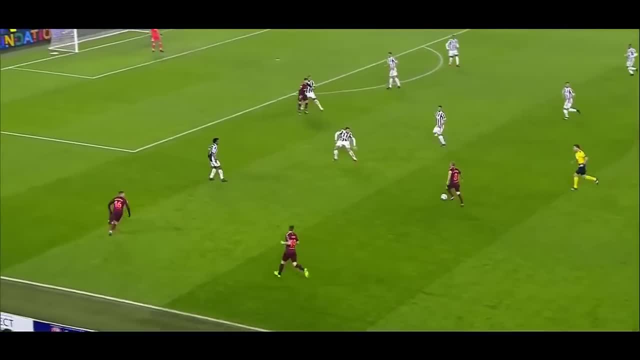 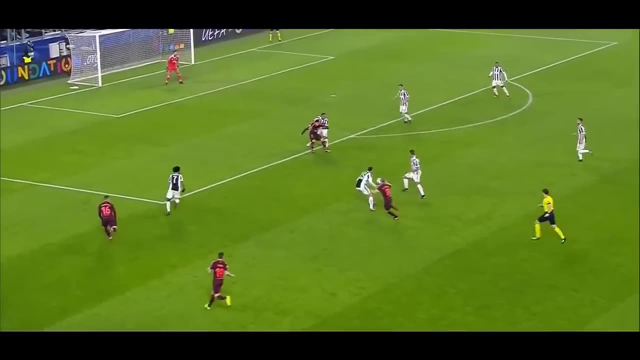 usually it's the right option. here he is, he plays it into suarez. it's almost a really good play. suarez may be being held back again, attack minded, but look at how he moves after the pass. again. you want to pass and move all the time in the midfield- gets the ball again in plenty of space. 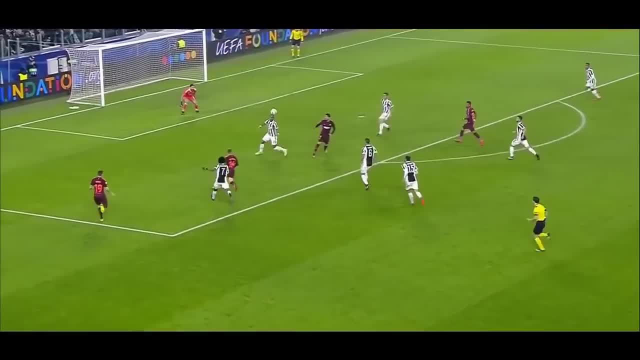 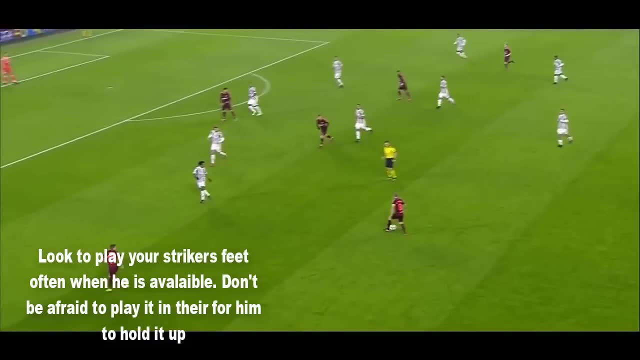 and plays really a really good ball, and then suarez kind of messes that play up it's a great ball into suarez. the other player from barca runs off the ball, makes a really good run and i'm not sure why suarez popped that ball up. if he just played it on the ground they would. 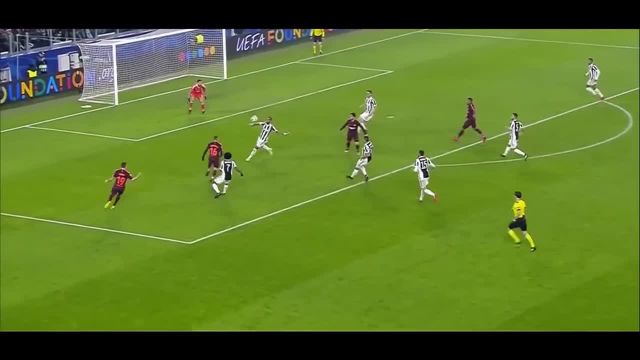 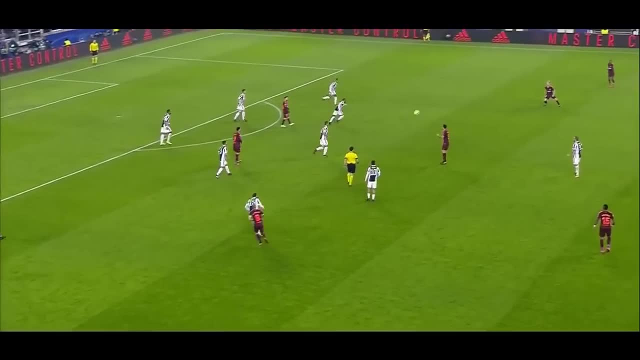 have probably had a good goal scoring chance, but by any, esta, that's a great play again with the ball, a good little switch out wide, nothing more to it. but again, always be looking to switch the field when the options available and especially when it's congested on your side. so here he is. 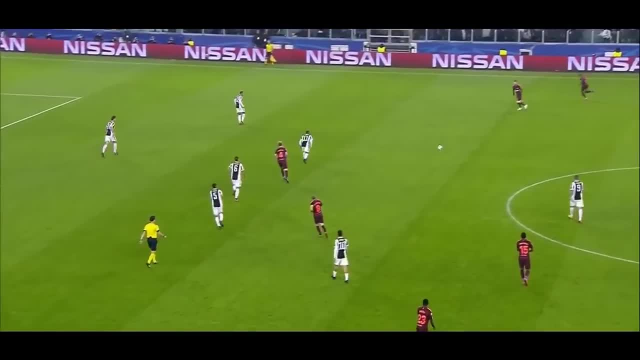 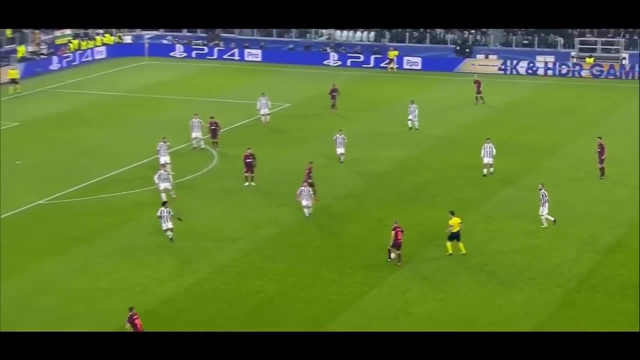 again. just simple: play out wide. nothing more to that one here again in so much space and he's got. he's just going to keep the ball a little bit and then play it out wide again. nothing too fancy, just moving the ball around and keeping possession here. he checks to the ball very well, does really. 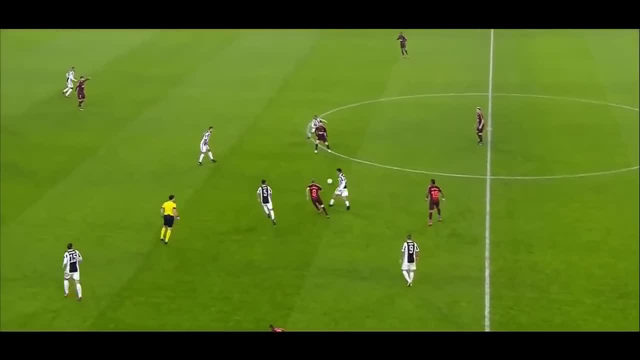 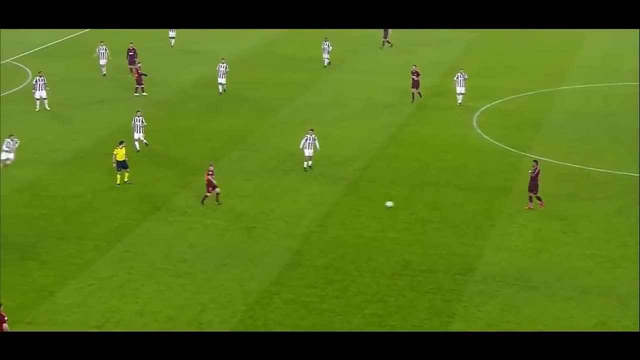 well to keep possession, they get the advantage and again, just kept moving it. here he's getting the ball in great space. great move, great awareness, knowing that the defender is in great touch and then plays it out wide. this is another great play. it's a great run by iniesta and his touch is just. 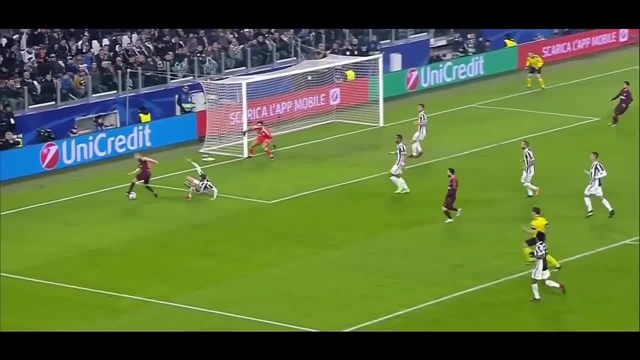 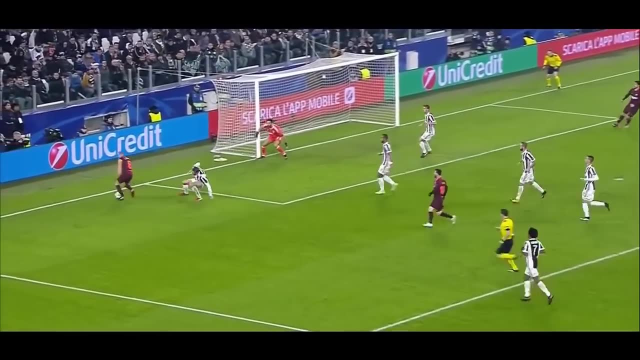 he has is he's trying to take a first touch out wide, giving himself enough space between himself and the defender to get a shot off. the defender just does a good job and then, uh, forces iniesta to give the ball up. but i think it's the right idea. by anyesta he may be able to shoot first. 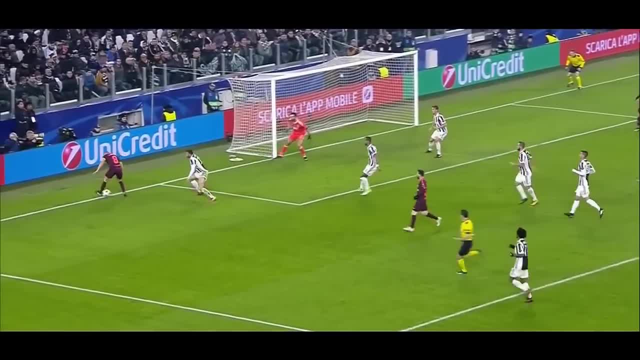 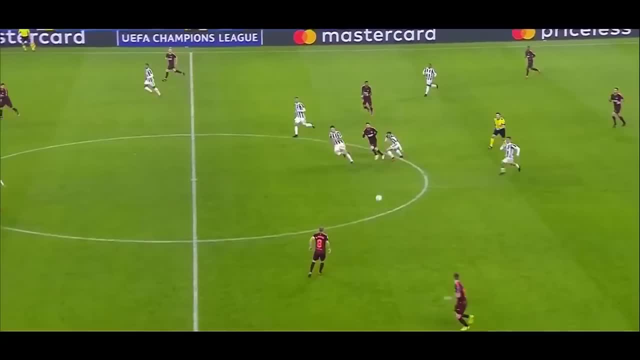 time here, but i can understand he's trying to give himself a better opportunity in this play. so here again, in plenty of space, is going to be his last involvement. just plays it in the Suarez good idea who plays it out wide? and actually this is his last involvement. great first touch takes the.